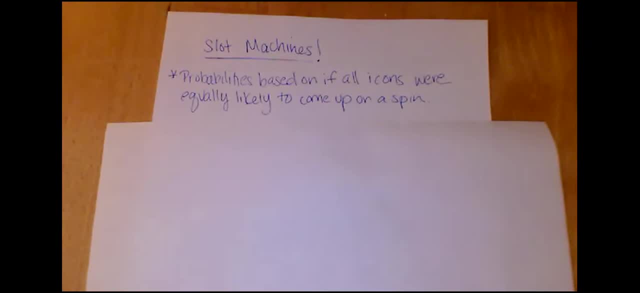 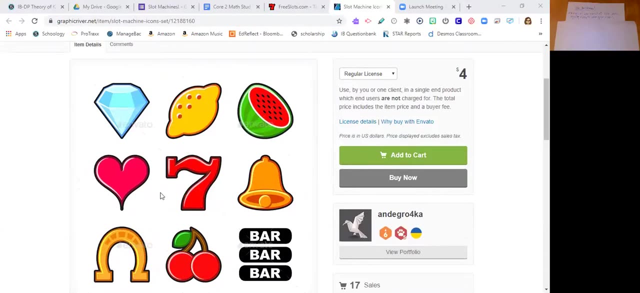 with you And so we can investigate what icons look like. So there are many different icons on slot machines, So these are the icons, the kind of the standard ones. A lot of people say that when triple sevens come up, that's a great sign because you won the jackpot. Sometimes, if cherries 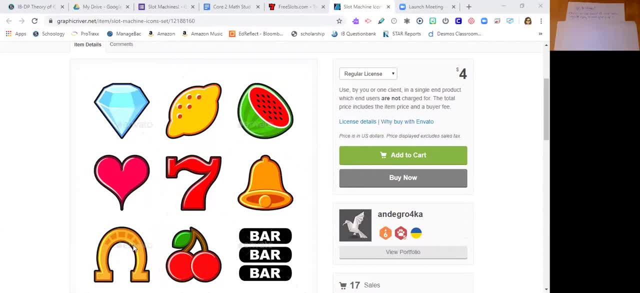 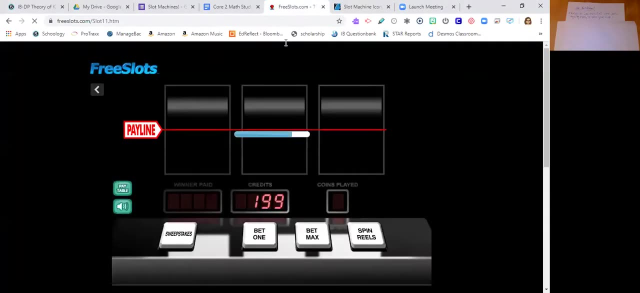 comes up or the bars come up, You win things too, And, of course, the lucky horse show. So what do I mean by coming up or being lucky or things like that? So let me show you. Here is it's called free slots And, yes, you can play for free. This is kind of a virtual 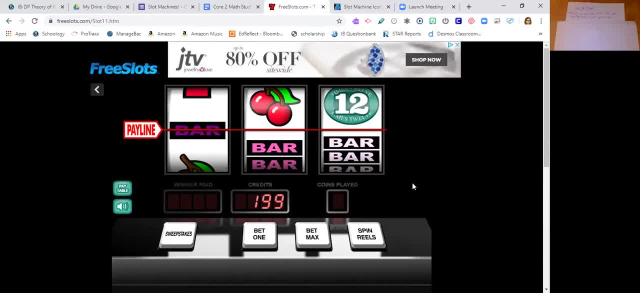 slot machine. This is something that you would see on when you were at a casino Down here. actually, here this is the pay line, So when it lands on this line, then what it lands on, you can get paid a certain amount of coins or money. Here they're. 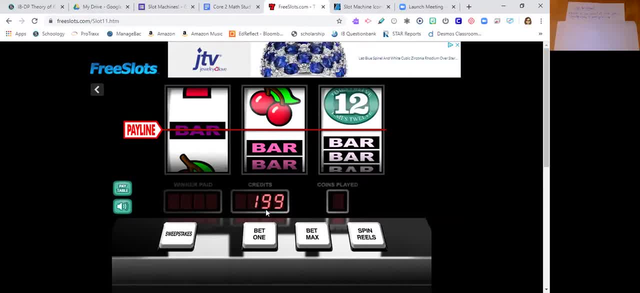 called credits, And so you can see I have 199 credits. We're playing penny slots- that would be 199 pennies. We're playing dollar slots- that probably $199.. So, depending on what kind of slot you want to play, that's what the credits are going to be based upon. Now we can bet one or bet max. 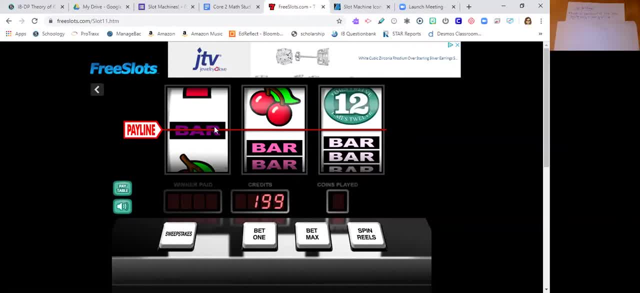 Here's your spin reels. So that's going to spin this wheel, that's going to spin this wheel and that's going to spin this last wheel. So right now, I'm just going to bet one, So I'm playing one coin, whether that. 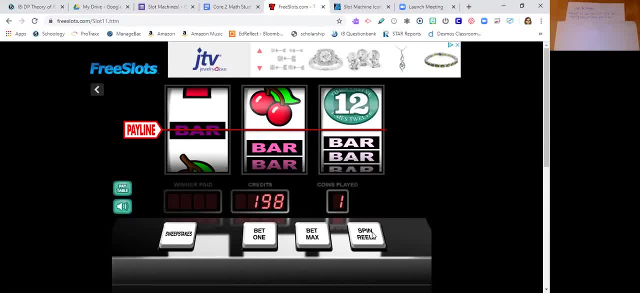 be a dollar, a quarter, five dollars, but I'm just doing one, I'm going to spin my wheels. Oh so, because I got that combination of double bar, then a single bar and another single bar, I actually won five. 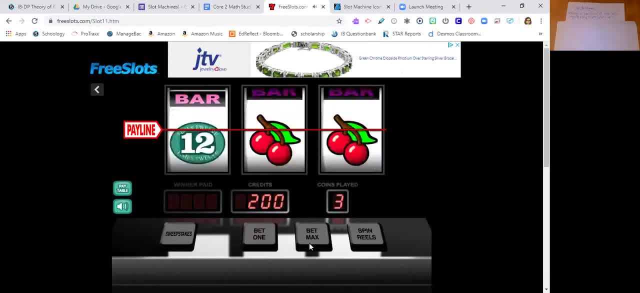 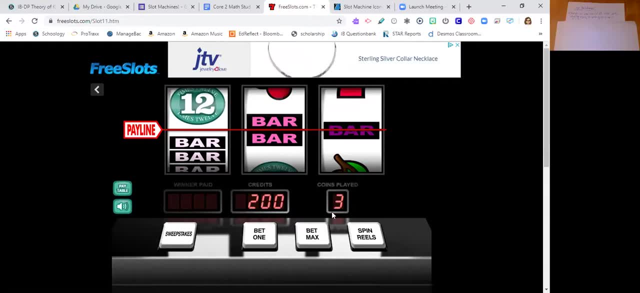 That's pretty good. I'm wondering what a max bet is. Okay, so max bet you can say three coins. I had a play, I played three coins and I didn't win anything, So maybe I'll go back betting one. 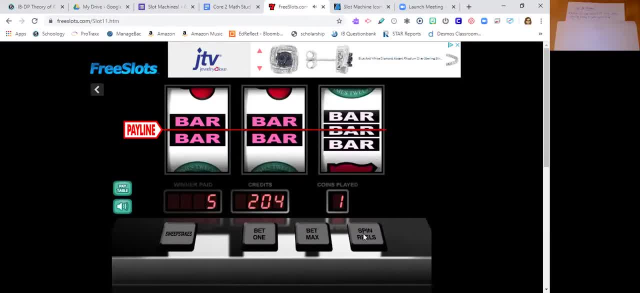 for me to back down to 199.. Let's see here: Wow, that's pretty good. So this is how you play: you bet one or bet the max, and then you spin the reels Here. this is your pay line, So whatever. 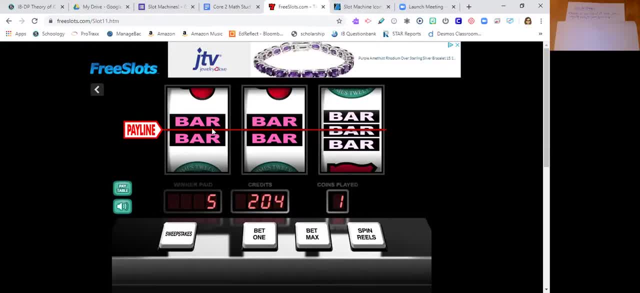 you're betting on here triple sevens, as you can see, a seven. if a seven and a seven and another seven came up, you win like a jackpot. So it's always exciting to do. Okay, so that's how. slot. 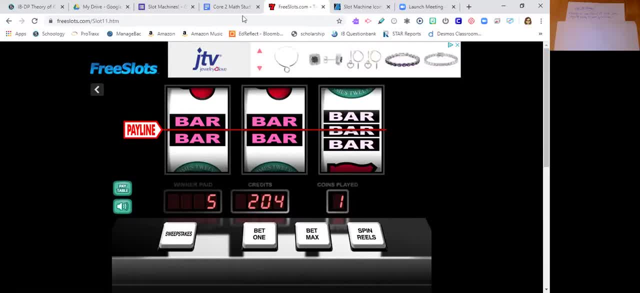 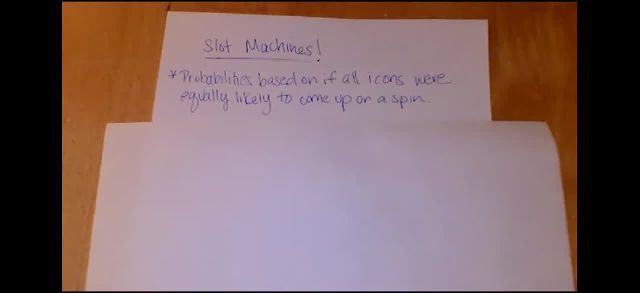 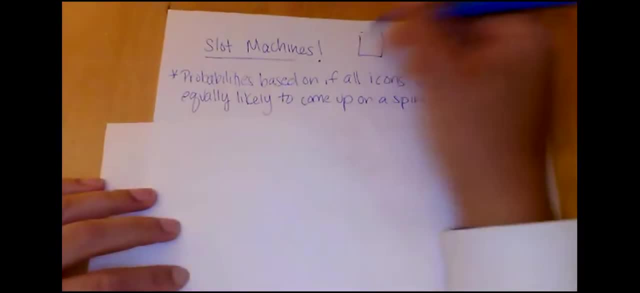 machines work. Let's go back now and look at some of the probabilities. So, as I said before my disclaimer, these probabilities are on if all the icons were equally likely to come up. So if that double bar was equally likely to come up on that first little reel and it was equally 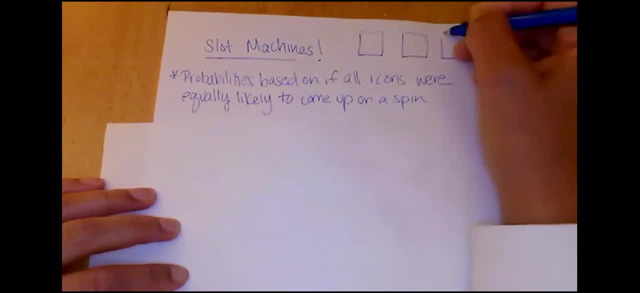 likely to come up on that second, as it was equally likely to come up on that third. Well, what do I mean by equally likely? For this game, there were nine little pictures, which we called icons. There were nine pictures that could have come up in the first reel. there were nine pictures. 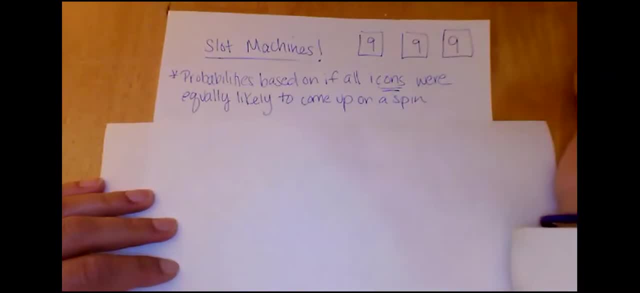 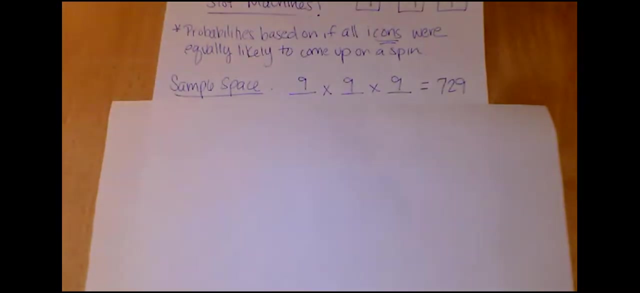 that could have come up in the second, and there were nine little pictures that could come up on the third. So each one of these reels, the pictures, are equally likely to come up. they have the same probability to come up on the third. So let's take a look at what I mean. First, we have to 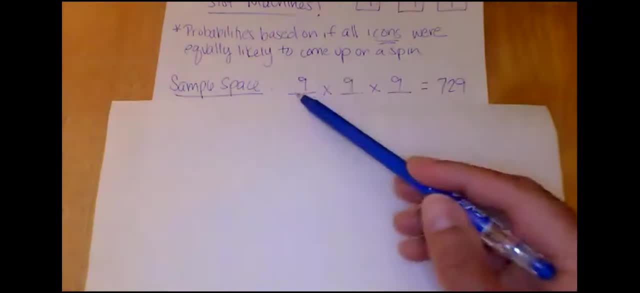 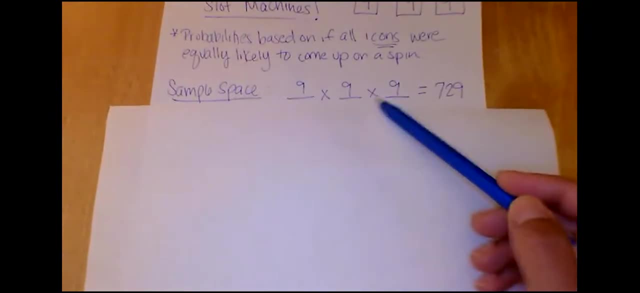 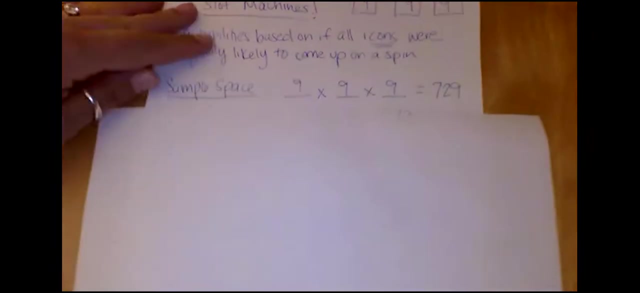 investigate our sample space. How many total combinations can there be? Well, there's nine possible icons in the first and multiplication nine on the second and multiplication nine on the third. That gives us 729 combinations. Well, here we have. total outcomes: 729. 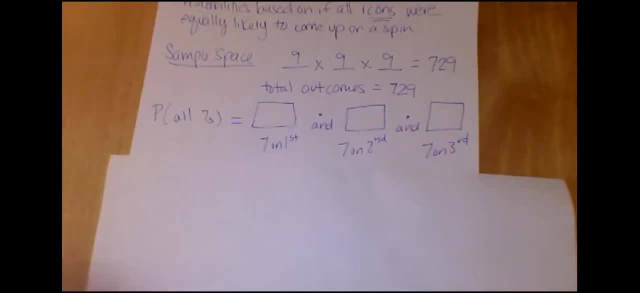 So let's take a look at what I mean. First, we have to investigate our sample space. How many total combinations can there be? Well, there's nine possible examples. Well, here we have total combinations for each: ie: n equals six. where n equals three. where n equals кв, where n is equal to the number of. 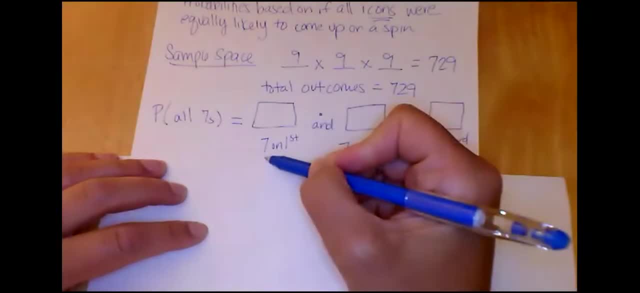 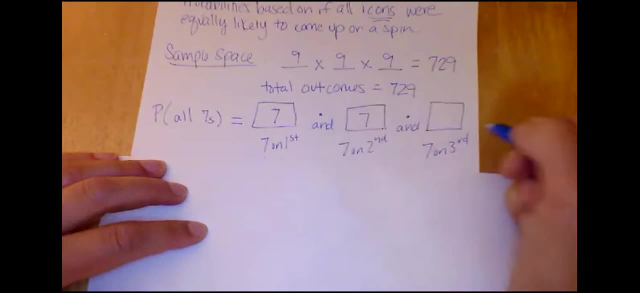 j, We have total level. Let's say that we have our sample space, number five. Let's say, if we want to play, we want to win the jackpot, So we're playing for all sevens. So let's find the probability of getting all sevens. Right now we have to. We want the probability of getting all. 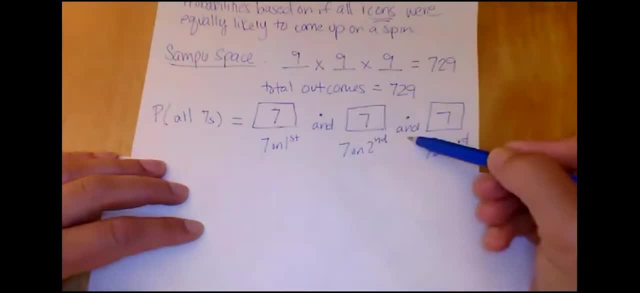 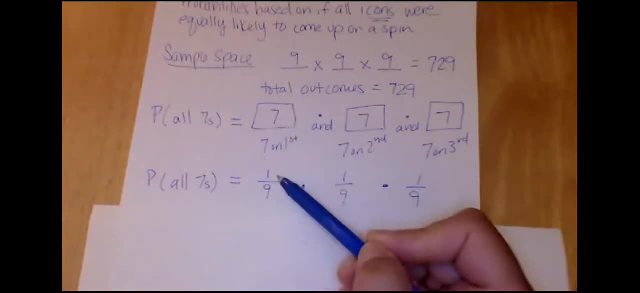 sevens acquired. Let's say that I want a seven on my first real. seven has to pop up And I want there is one seven out of nine on this first real. so that's what I mean by equally likely. the second one, again, there's only one seven out of nine. 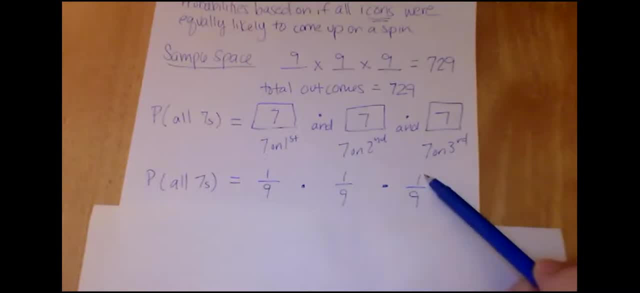 possible icons and on the third there's only one- seven- out of nine possible outcomes. so the seven has a one out of nine chance to come up on each of these reels. that's what I mean by equally likely to come up. so if we have all sevens, that means I need the first one and the second one and the third one. so 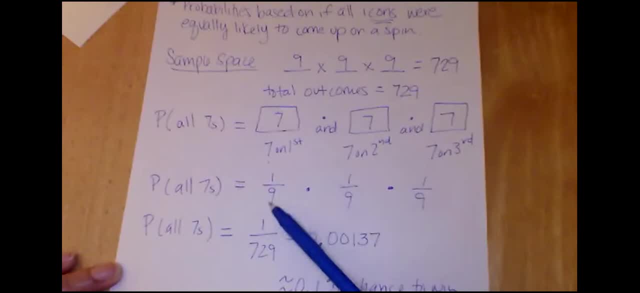 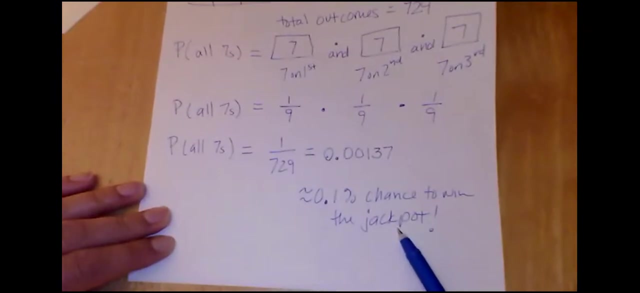 I am multiplying one times, one times one. this one nine times nine times nine gives our total outcome seven hundred twenty nine. so that gives me a point zero, zero, one, three, seven probability, that is about point one percent chance to win that big jackpot. done, done, that is a very, very low. 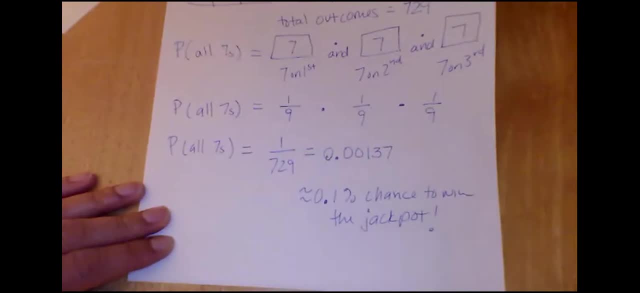 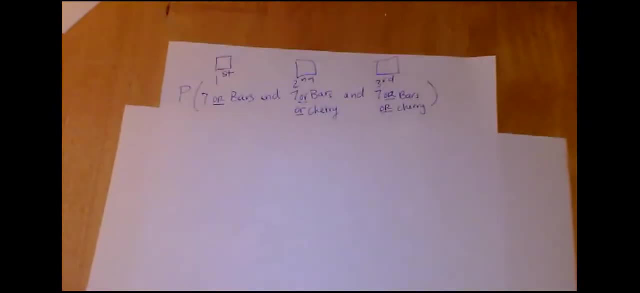 probability, still a chance, very low probability. so let's take a look at combinations. so, as you saw, there were some combinations. so sometimes those triple bars came up. so you know, or you can get a single bar, sometimes cherries can come up. sometimes you could have like a seven on the first, a bar on the second and a cherry on the third. So any. 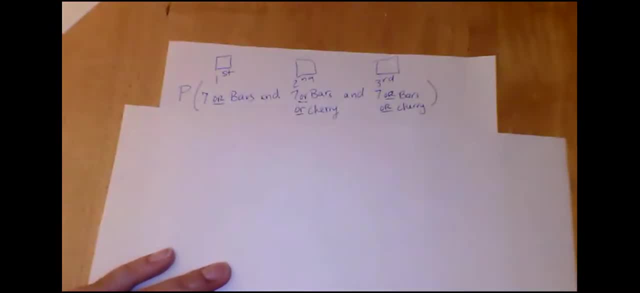 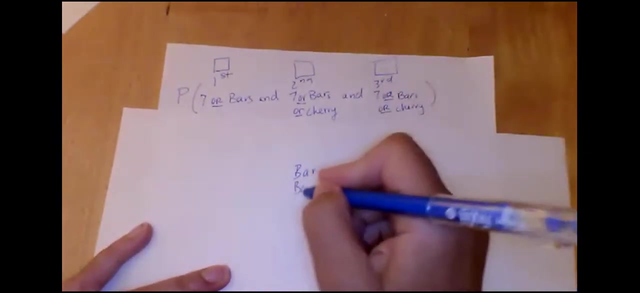 one of these types of combinations can come up, You can win some money. So you don't just need to get all sevens to win money, It's just all sevens mean to win the jackpot. So, like you saw on, that's my last spin. I actually had whoops. my last spin I had a bar on the first bar bar. 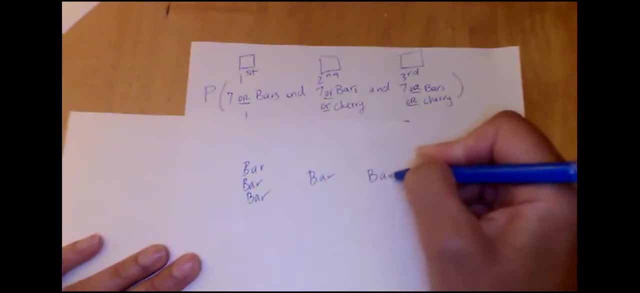 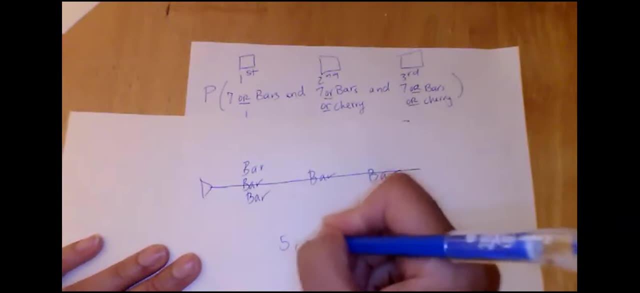 bar on the first, and then I had a bar on the second and I had a bar on the third. So, and here was my little win line, And so I won five credits. So this was one of the combinations. So there are. 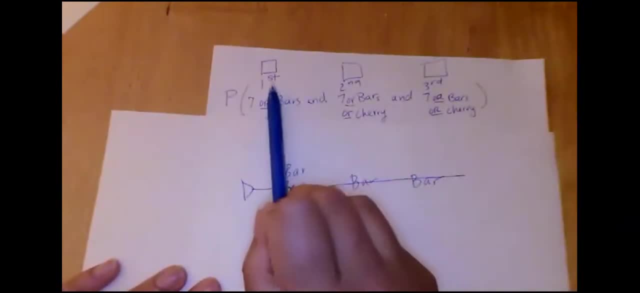 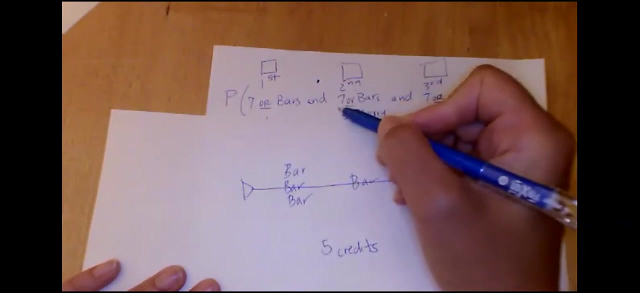 many different combinations And I picked out one combination here, So my first one. I can say, let's go to find this probability that on the first one either a seven or the bar comes up And multiplication On the second one, let's say that a seven or a bar or cherry comes up. Okay, So that's, that's fine. 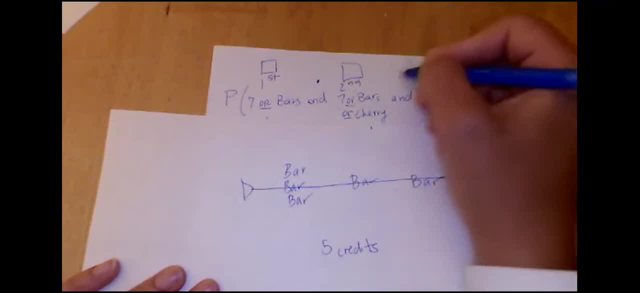 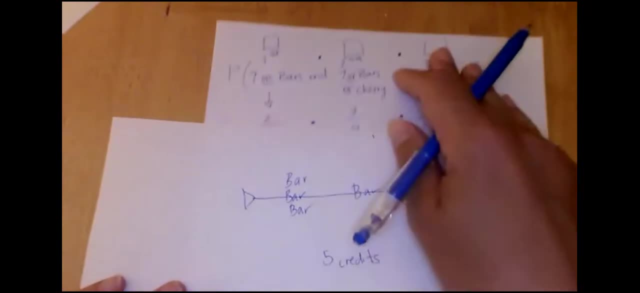 I don't, whatever combination comes up, it's going to be a winner. And multiplication. On the third, a seven or a bar or a cherry can come up, So let's find the probability Okay. So on this first one, 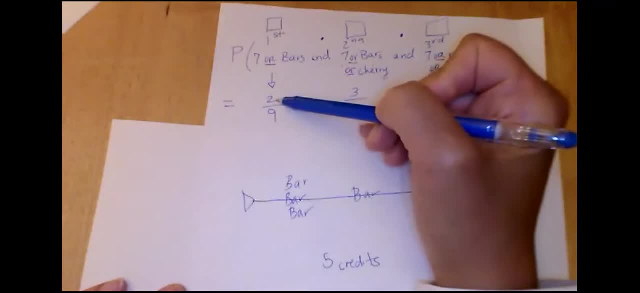 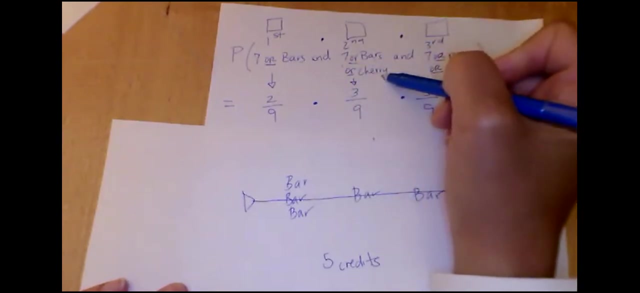 there's a seven or a bar. That means that there's two, one, two out of nine total icons that can come up when I spin, Okay, And on my second one I could have a seven or a bars or a cherry now. So now I have three different possible ways out of nine, So that's a three out. 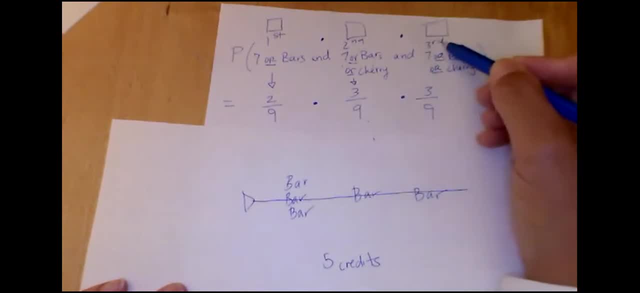 of nine And multiplication On my third one I could also have a seven or bars or a cherry. So one, two, three possibles that I can win out of nine. So here my probability gets a little bit better. Let's see how much better it actually gets. 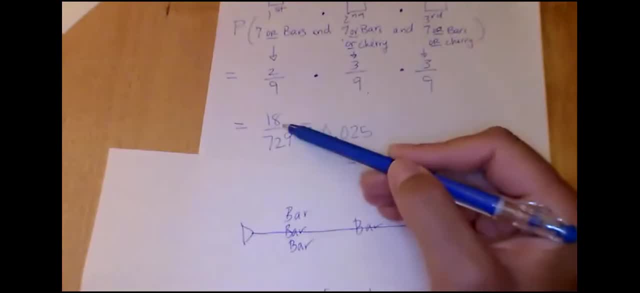 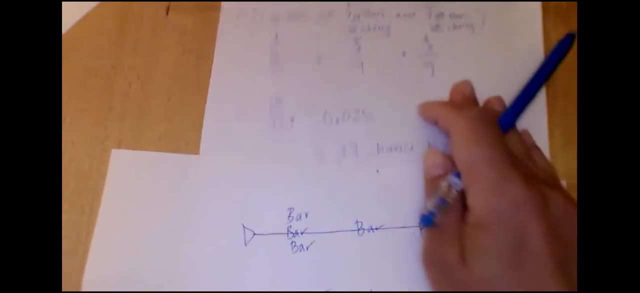 Okay, If I multiply two times three times three, I get 18.. Of course, nine times nine times nine is 729.. That means I have a probability of 0.025.. That's about a 3% chance to win some money. 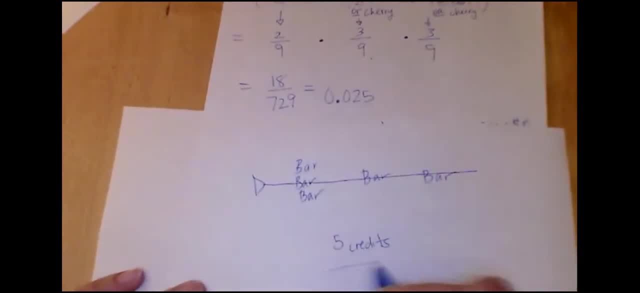 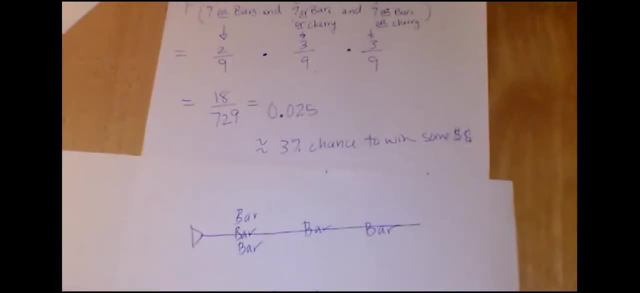 Maybe it could be five credits, like I've won down here, Maybe it could be two, Maybe it could be one, But still a very small probability than what we've been used to learning about our other types of games of chances, like roulette. So here's the trick that the casinos use Now: probability of winning the 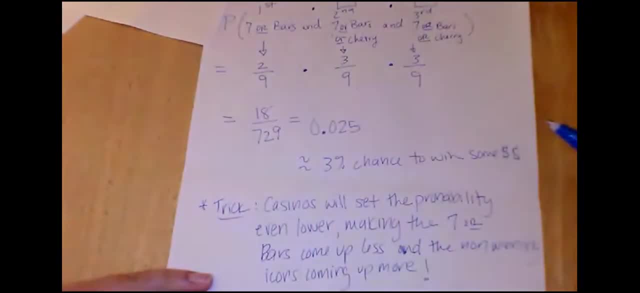 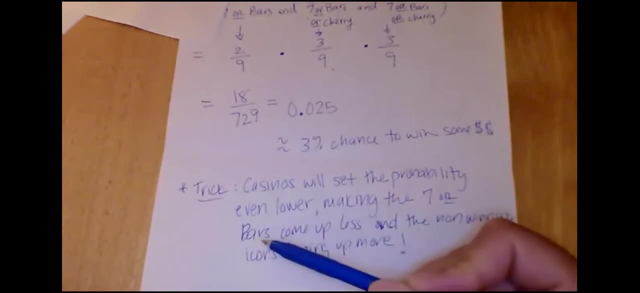 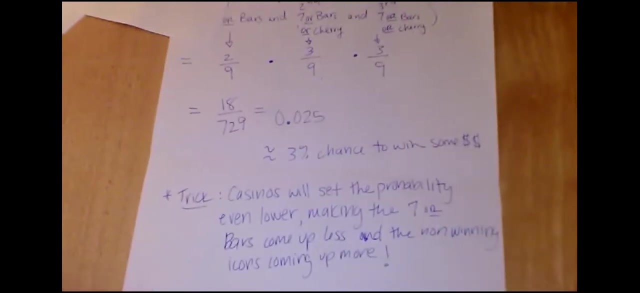 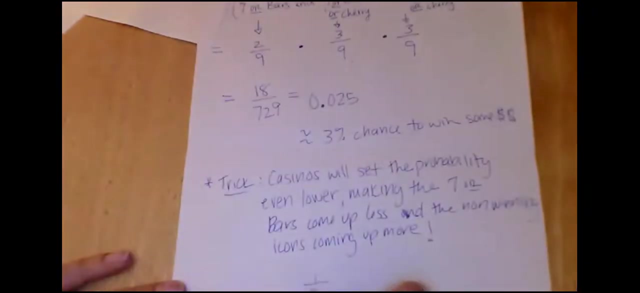 jackpot very low. Probability of even doing combinations very low. But the casinos will set the probability even lower, making the seven or the bars come up less and the non-winning icons come up more. So the seven: they might set the seven to come up on that first one, like maybe one in 100 times. not just one in nine, They might set it to one in 100, just on that very first slot there. So that's what happens with casinos. So you think you're winning, you're winning, but that's maybe just because it came up on that. 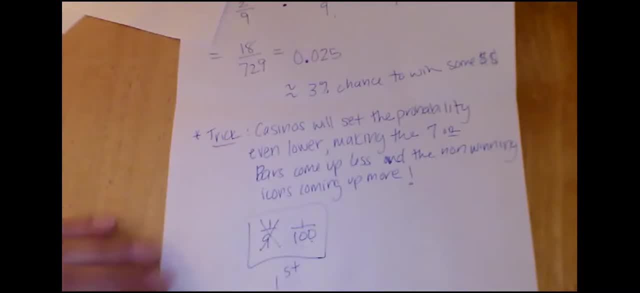 You're that 100th person that spun that wheel, or that you gave it that 100th spin, not the 100th, the 100th spin- and it actually came up for you. That means that there's probably going to be 100 more spins. you're going to have to wait So they won't set it to. equally likely.